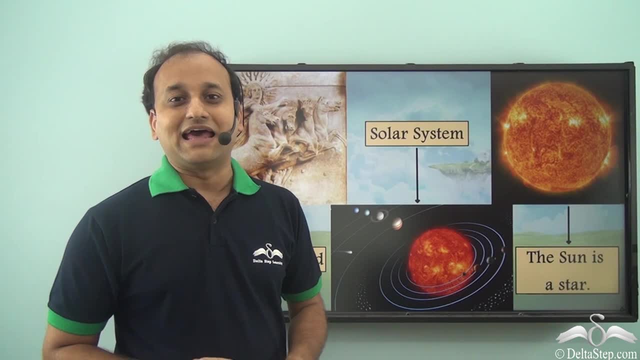 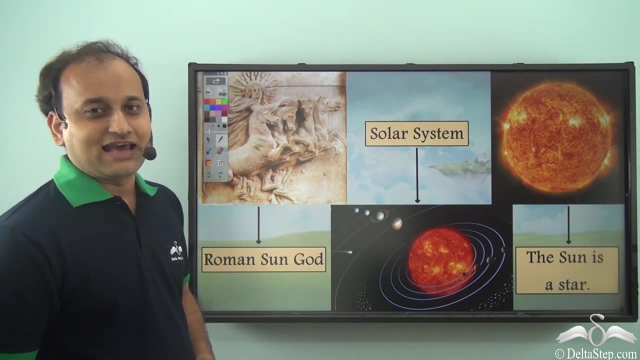 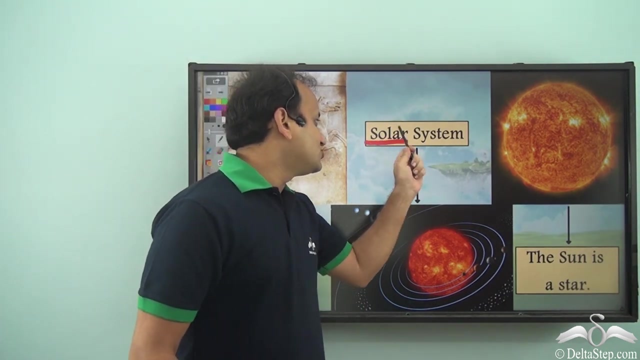 that is why scientists have given it a name, And that name is Sol, which is the name of the Roman sun, god, And that is why sun is called Sol by scientists, And from Sol comes the word solar And the planet system which revolves around the sun, it's called the solar. 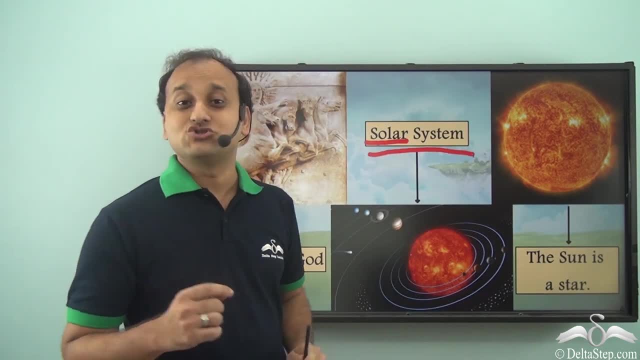 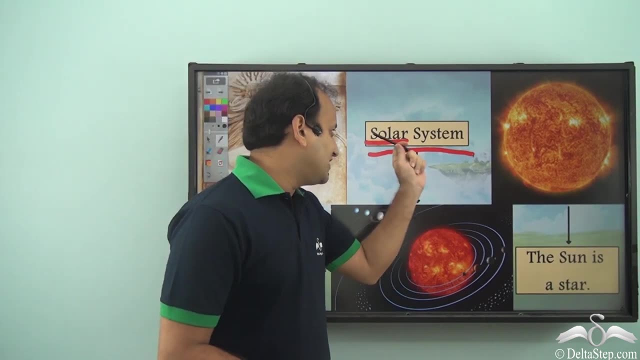 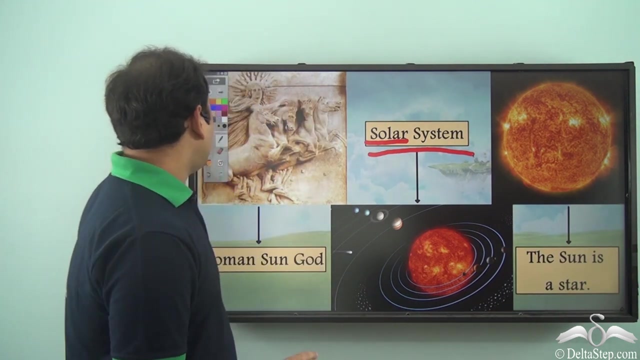 system because it's Sol's family solar system. Okay, so now we know that the head of the family is sun, and why the name solar system. So now let's know the eight members of the family closely. So let's know the first member. 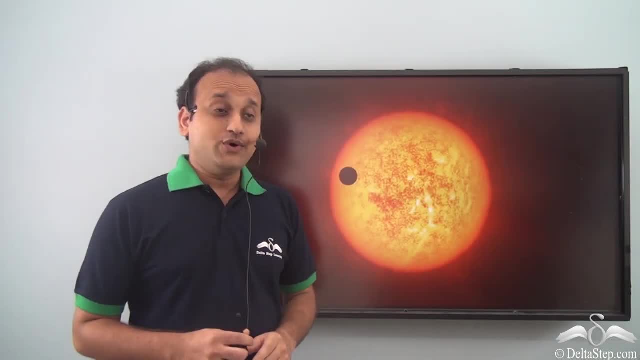 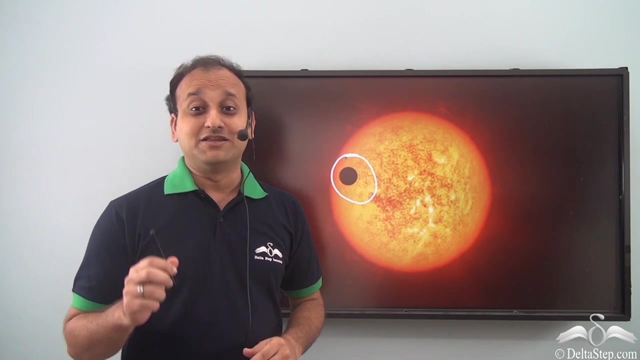 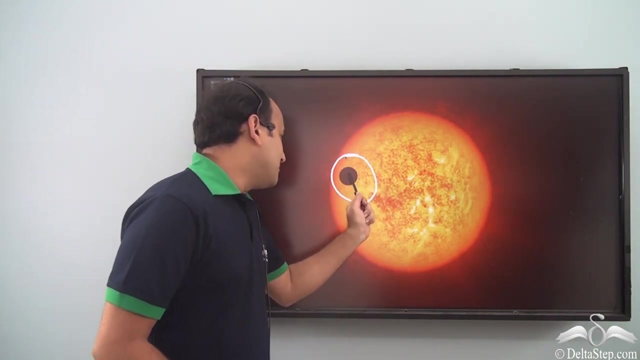 of the family, which is also the smallest. So the closest to the sun is the planet Mercury. It is the smallest in the solar system. You know, just like the smallest member in our family is the dearest to all and the mother always keeps that member closest to her, Similarly the sun keeps the Mercury closest to it. 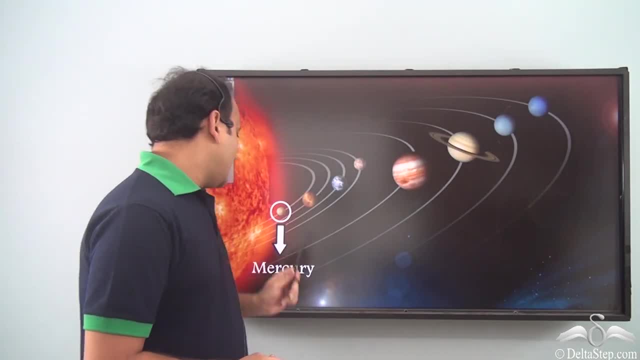 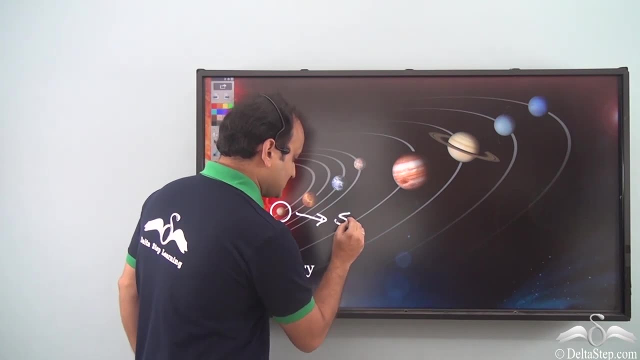 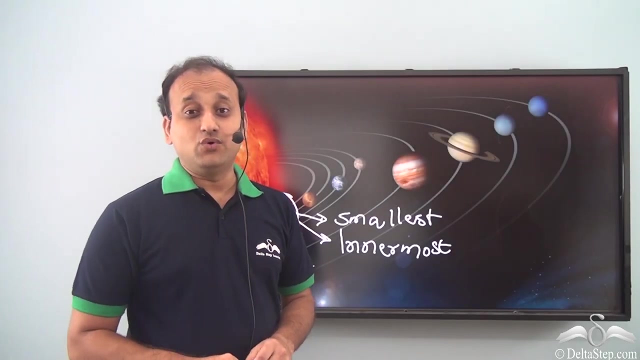 You see, it is the closest to sun And also Mercury is the innermost planet. that is, Mercury is the smallest As well as the innermost. So Mercury is the smallest and innermost planet of the solar system. So now that we know that, 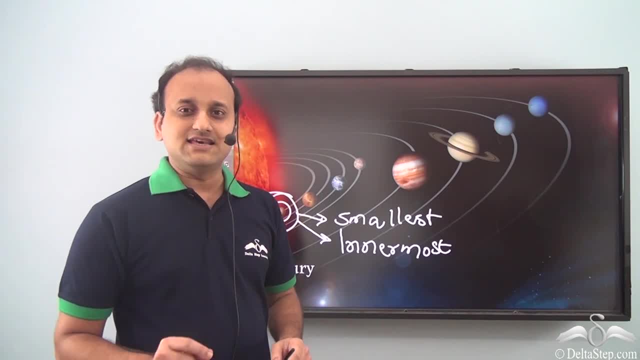 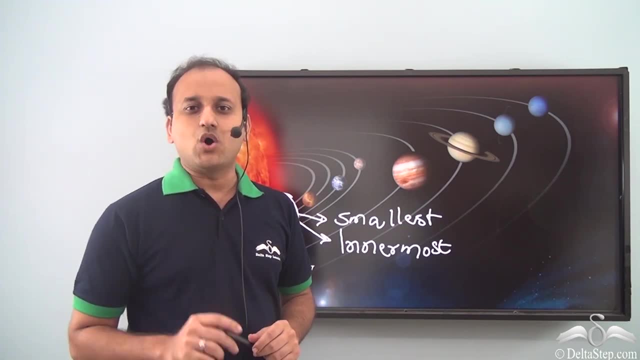 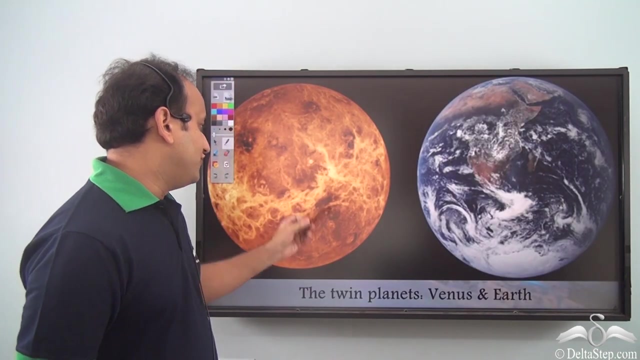 Mercury is the innermost planet of the solar system. let's see second in line, that is Venus. Now, Venus is very special in the solar system. Why? Because it resembles Mercury. Okay, Because Venus is someone who is very close to us. Let's see whom Venus resembles Earth. 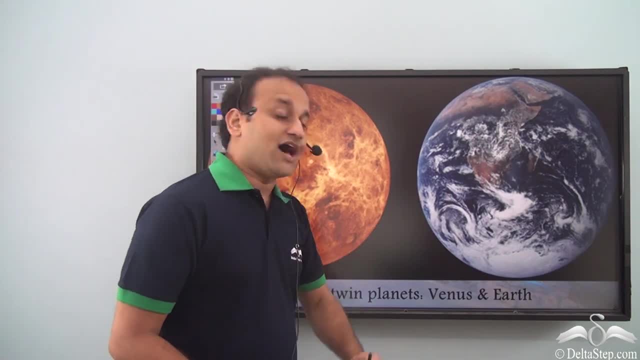 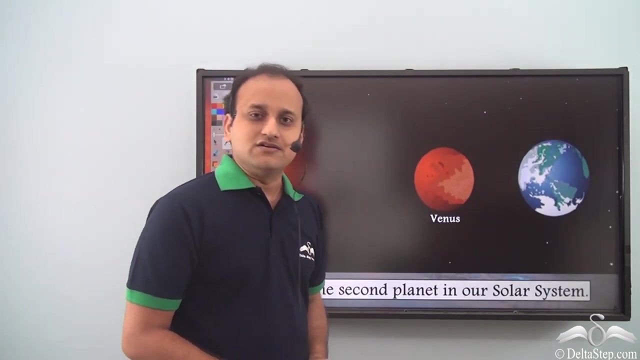 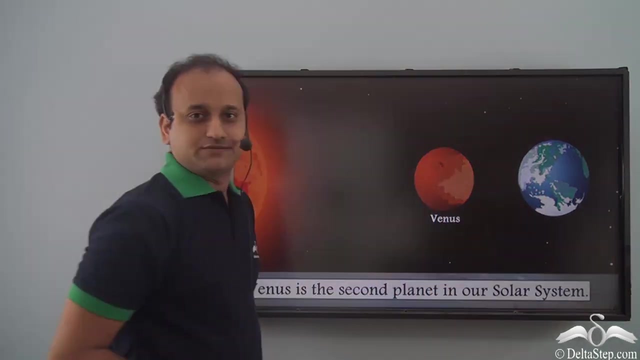 very much, And that is why both these planets are called twin planets, Because they have similar shape, similar size and similar weight. So these are called twin planets. Now, the planet Venus is the second planet in our solar system And it is just beside Earth. Now that we know Venus, let's know its twin planet. that is our home. 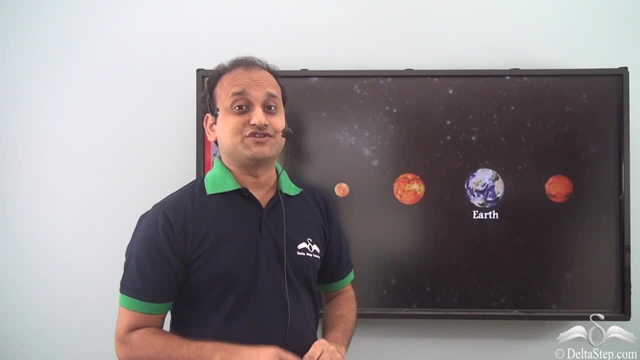 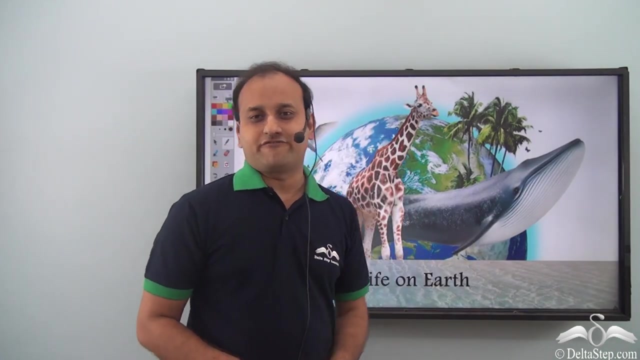 planet Earth. Now, the planet Earth, which is our planet, is third in line And it is one of the most unique planets in the solar system. So why is it unique? What do you think? Because planet Earth supports life, All the trees and human beings, the animals, the birds, the animals, the birds, the 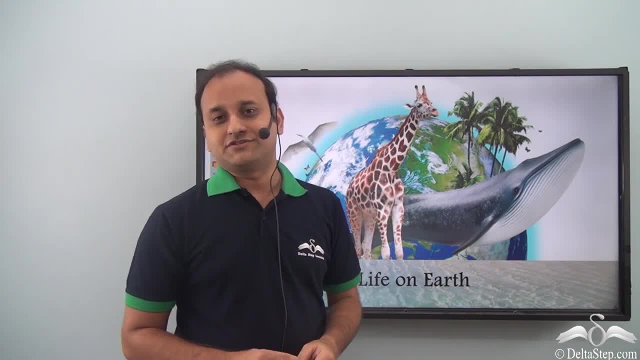 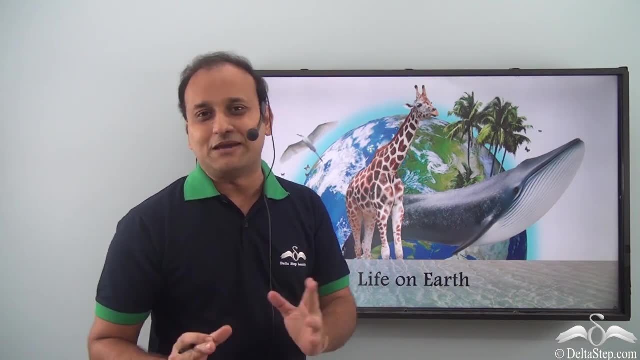 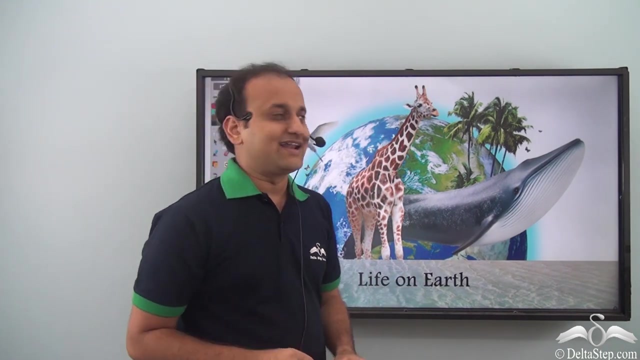 birds, the butterflies- all are there only on planet Earth. No other planet in the solar system supports life And that is why our planet Earth is a very unique planet. So we know about Earth. Let's know. the next in line, That is the angry young man of the family. You know, Mars is the 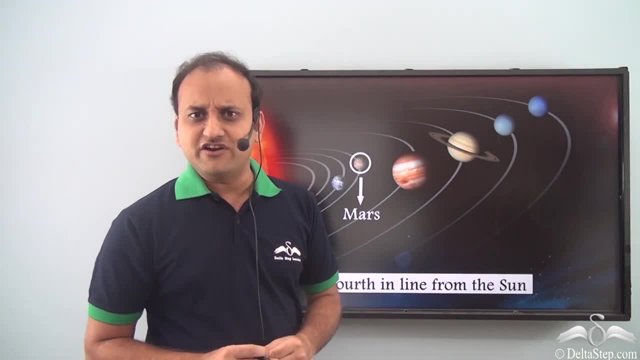 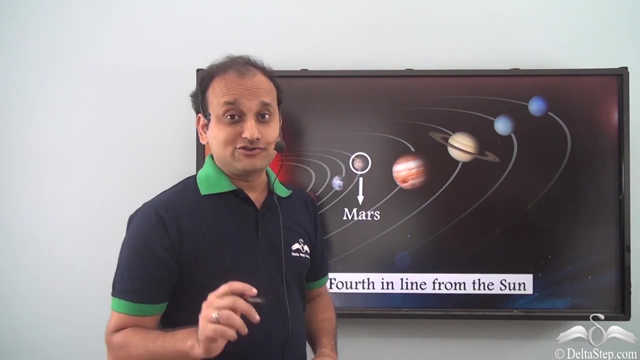 angry young man of the family. Just like when somebody gets angry, their faces go red, That's. you know, it's always red in color. that is the reason why it is known as the red planet. so once we know about Mars, which is fourth in line, it is also the second. 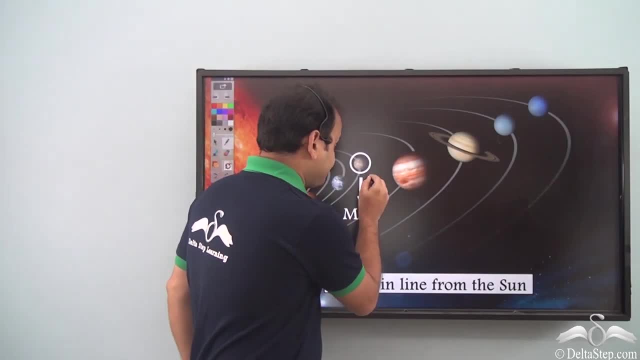 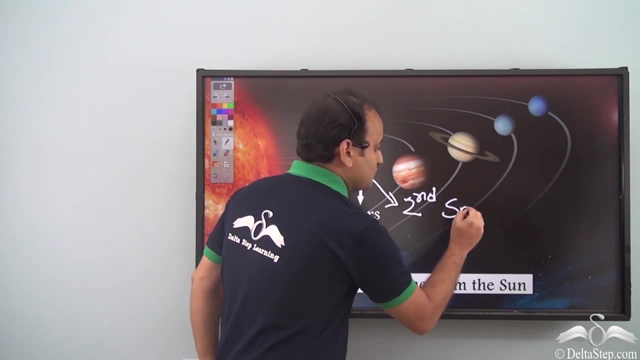 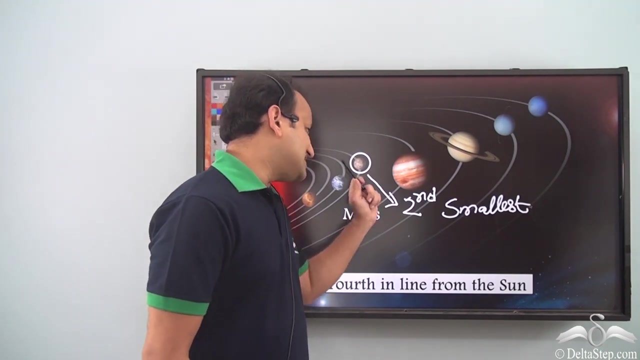 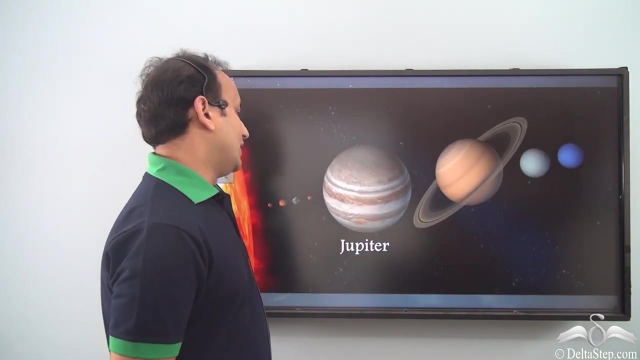 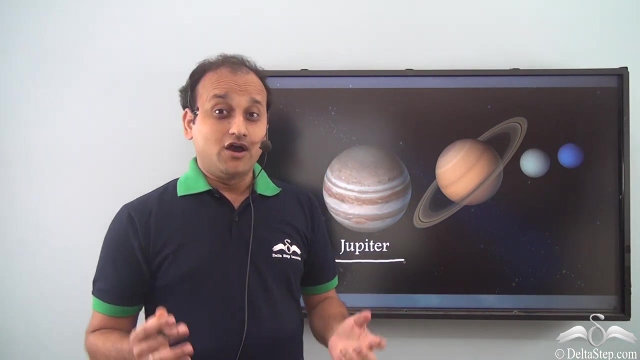 smallest planet of the solar system. so Mars is the second smallest in the solar system. now that we know the second smallest, let's know the biggest in the solar system, the largest planet. well, the largest planet in the solar system is none other than Jupiter, just like we have elder brothers who are the biggest. 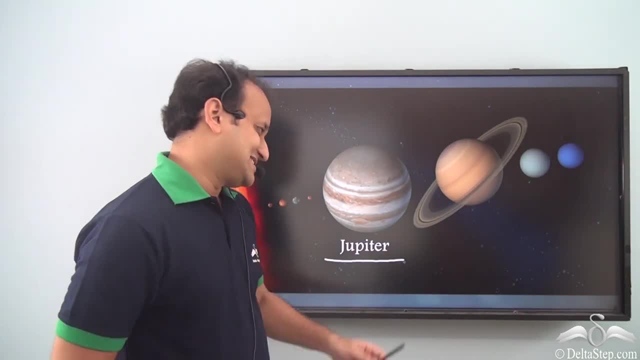 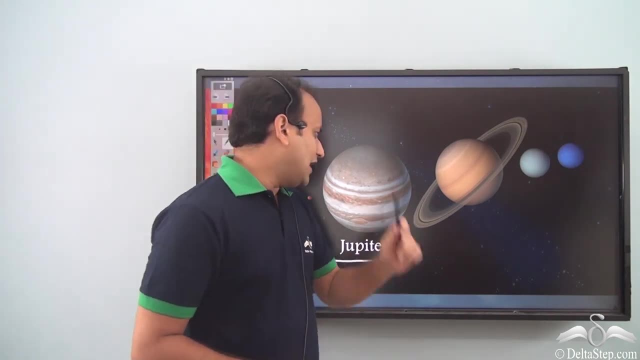 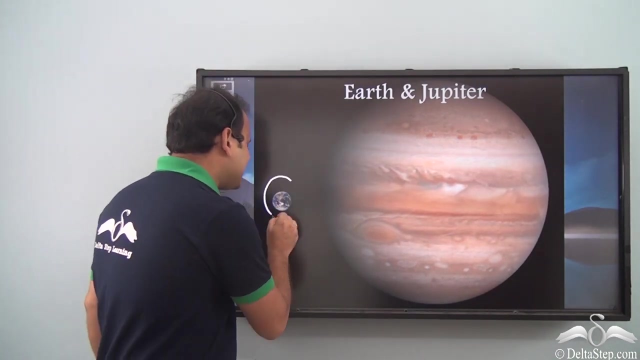 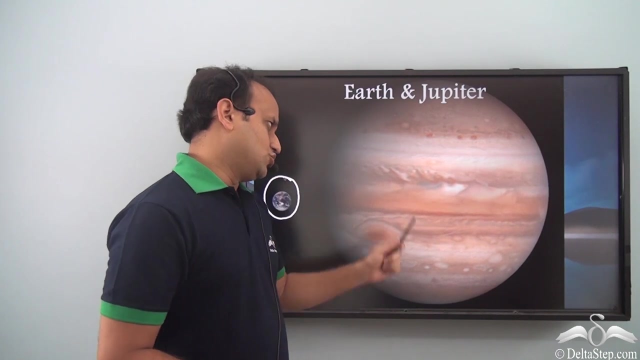 and strongest in our family and always take care of us. similarly, in solar system, that is Jupiter, the big brother of the solar system. now, Jupiter is so large that if you compare it to earth, it looks like a very tiny ball in front of Jupiter. such big and massive is Jupiter. so Jupiter is the largest in the 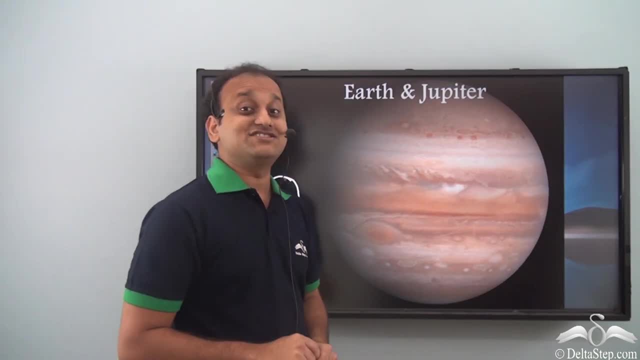 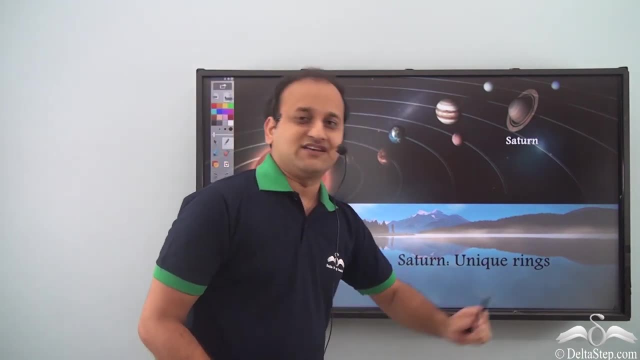 family, but who is the second largest? that is, Saturn. Saturn is the beauty queen of the family. it has its unique rings and it always likes to show it off, while even some other planets have their own rings and it always likes to show it off, while even some other planets 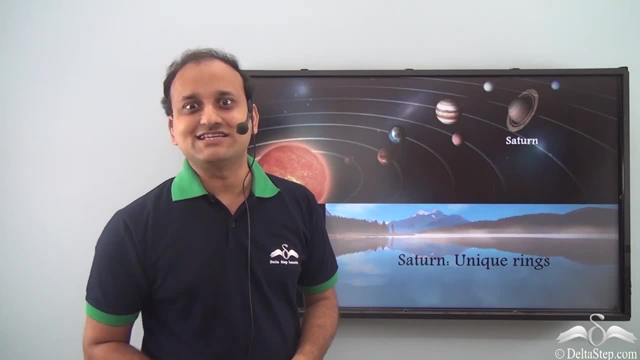 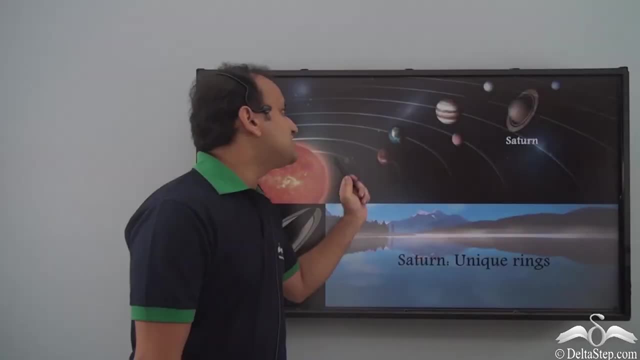 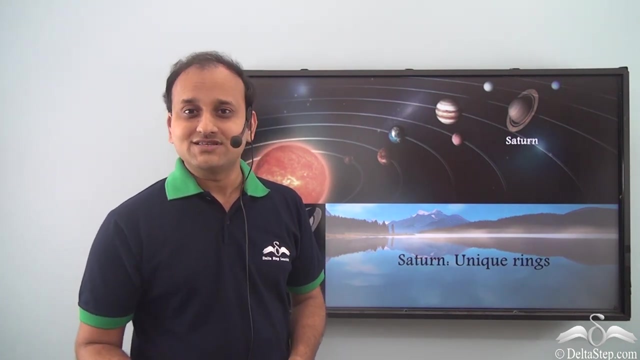 have rings, but they don't show it. you won't be able to see it at all, but Saturn is the beauty queen. it will always show off its rings. while Saturn is pretty far from the Sun, there are two more planets which are further away. those two are Uranus and Neptune. you know, they're like distant cousins just. 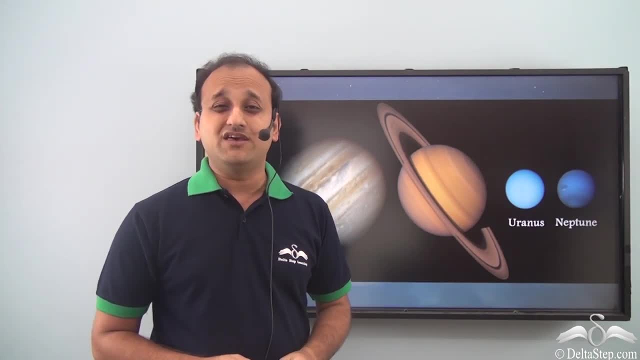 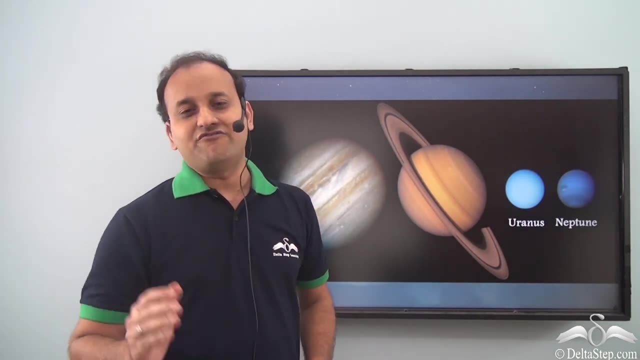 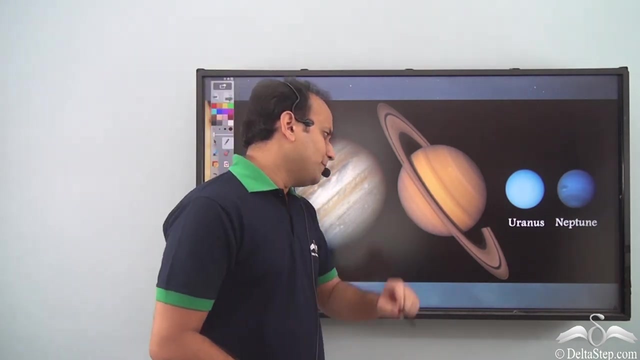 like. we have some distant cousins who live very far off and we meet them maybe once a year in family get-togethers. such are Uranus and Neptune. they are very far and if you want to see them, they can only be seen with the help of a telescope. so these 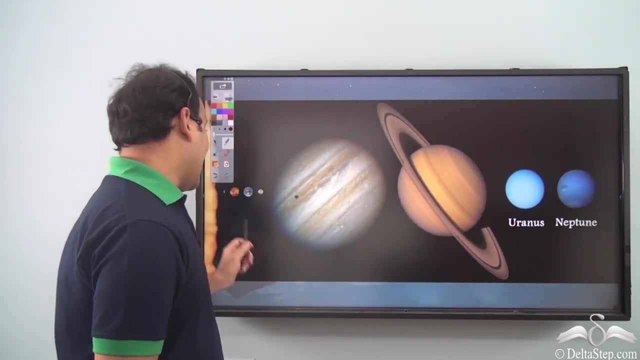 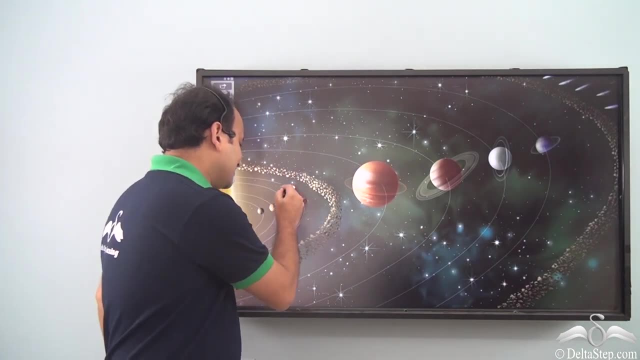 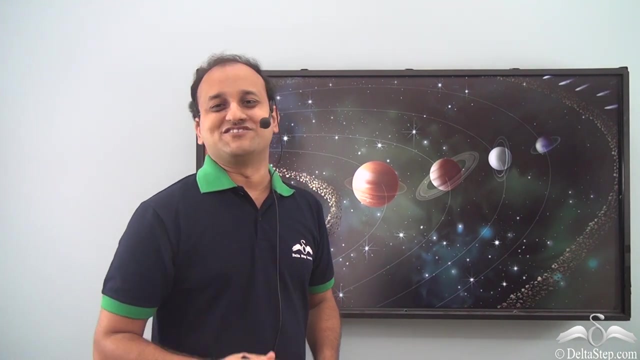 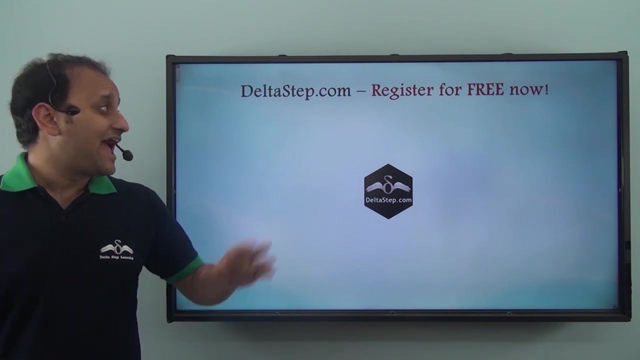 are the eight members of the solar system, along with Sun, the head of the family, and they all are part of our earth's family. so you see, our earth is not alone. it has a family of its own, which is called the solar system. don't forget to subscribe to our channel. you can also register for free at 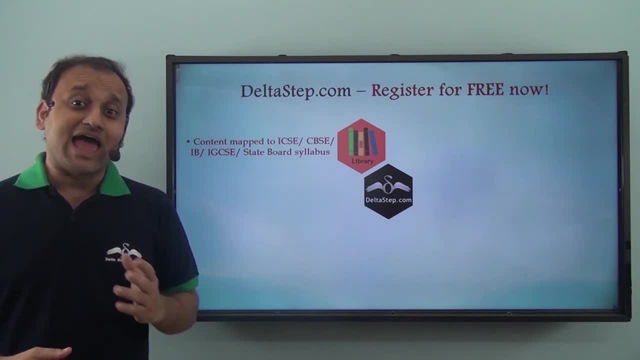 deltastepcom to get all learning resources as per ICSE, CBSE, IB, Cambridge or any other curriculum. over 5,000 amazing lectures across Maths, Science, English and Social Science. our unique interactive video technology keeps you engaged and our iDubbbz YouTube channel will keep you up to date with all our videos. Thank you. 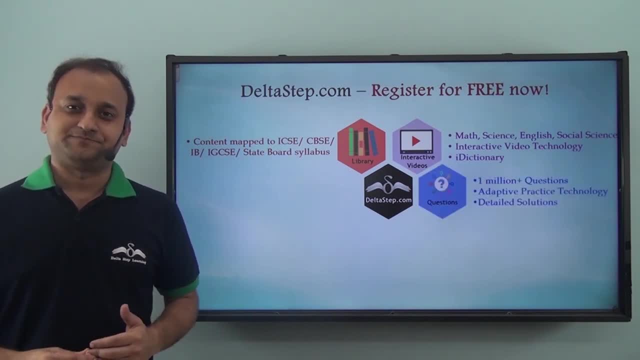 The iDubbbz dictionary feature allows you to quickly revise any concept. master each topic at your own pace with our adaptive practice technology and 1 million plus questions. get instant answers and detailed solutions. be exam ready by taking unlimited mock tests, performance analysis along with actionable feedback. 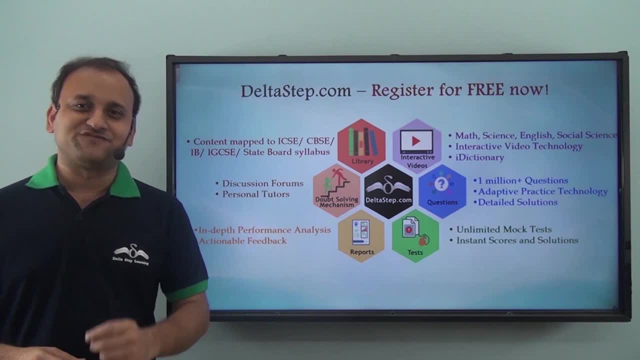 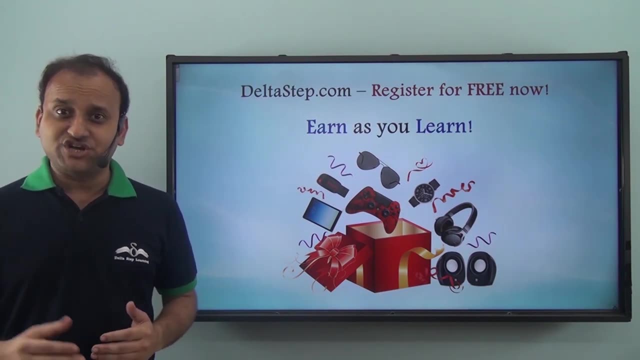 personal tutors to resolve your slightest of doubts. that's not all. you also get a amazing prizes like Playstations, iPads, watches and many more, along with certificates to our own as you learn program. so at deltastepcom, learning is not just fun and easy, it's rewarding too, so register for free now.